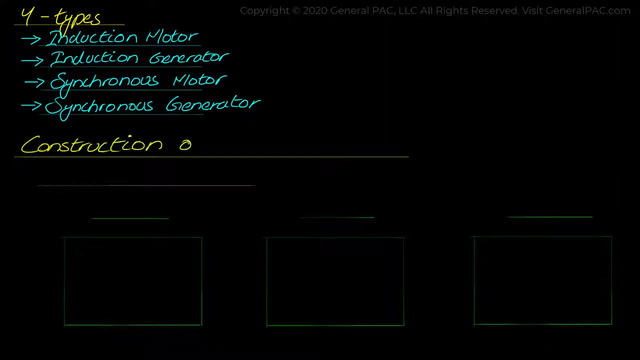 Now let's have a discussion on the general construction of an AC machine. Each 3-phase AC machine consists of two parts: We have the stator and we have the rotor. For the stator, which is the stationary part of the machine, it consists of a frame, core and 3-phase windings. 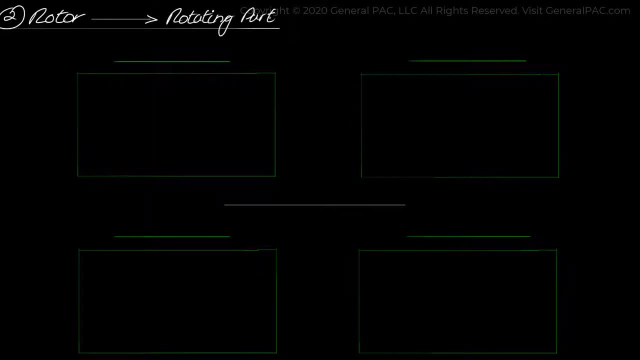 And for the rotor, the rotating part of the machines. these are two types of rotors in an induction. One is the squirrel cage rotor. It consists of conductor bars that are shorted, with end rings and a core in which the conductor bars are placed. 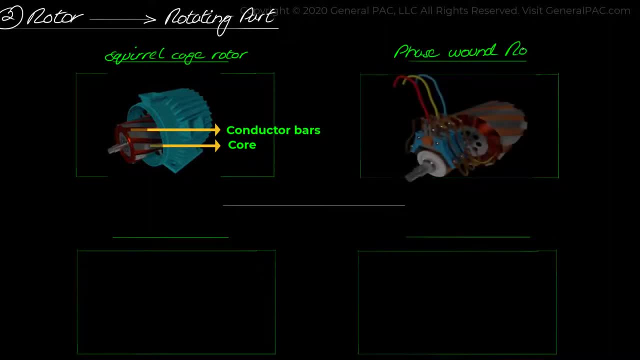 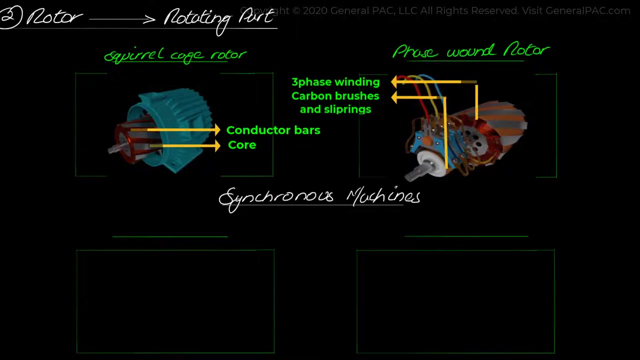 The other one is the phase wound motor, which consists of 3-phase windings similar to stator winding and has an option of adding external resistance through carbon brushes and slip rings. Also, there are two types of rotors in synchronous machines, Namely: 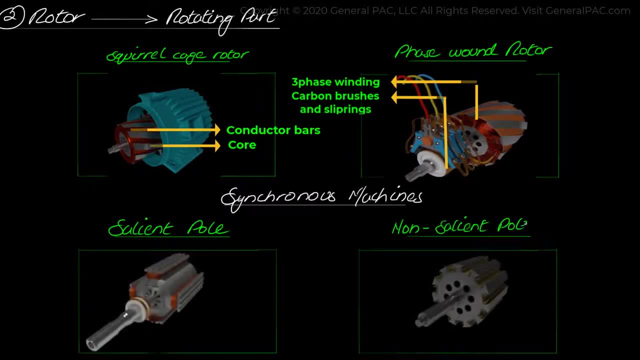 the salient and non-salient poles. The salient poles protrude out of the rotor and the non-salient poles do not protrude out of the rotor face. Now let's move on to the next area of construction and talk about the field and armature winding. 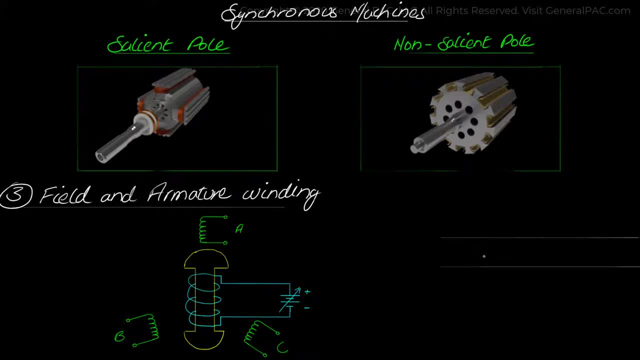 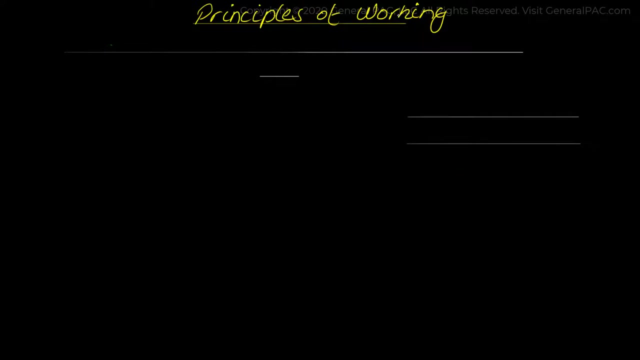 The concept of armature and field is related only to synchronous machines. Which is an armature is an AC machine in the stator winding, While field winding is constant DC supply provided at rotor. Now we're back. Now let's continue to have a quick idea about the principles on which AC machines work. 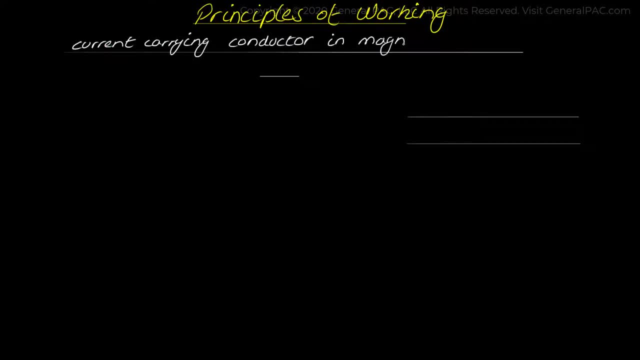 Whenever a current carrying conductor is placed within a magnetic field, a force acts upon it. The reason behind this force is due to the interaction of the magnetic field that is supplied and the magnetic field produced due to the current carrying conductor. If this conductor is arranged in order to form a line, 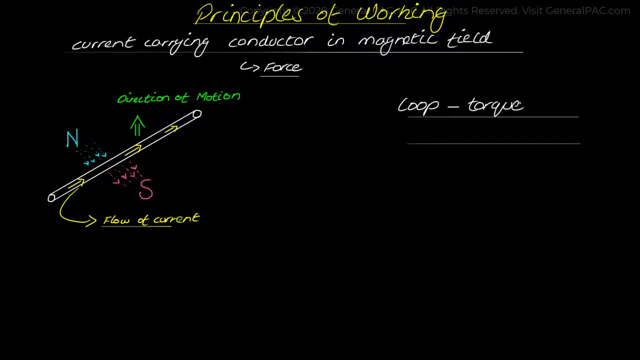 in order to form a loop, a torque is developed. due to the change in the direction of current, The torque will then move the coil in a circular path, hence creating the motor effect. Now let us connect this with a Motional EMF. 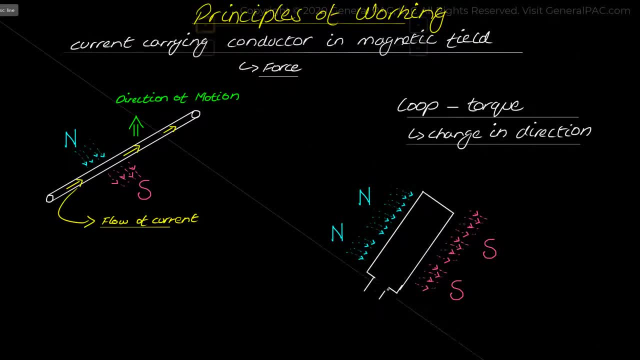 A Motional EMF is. whenever a conductor is placed in a changing magnetic field, It tends to have a voltage induced on it, and if it is formed in a closed loop, a current flows through it. a force acts upon it. The opposite is also possible. 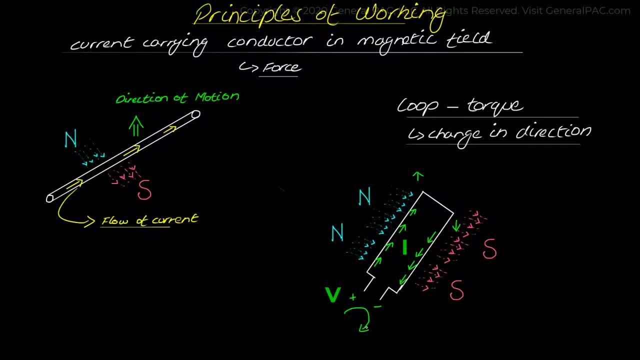 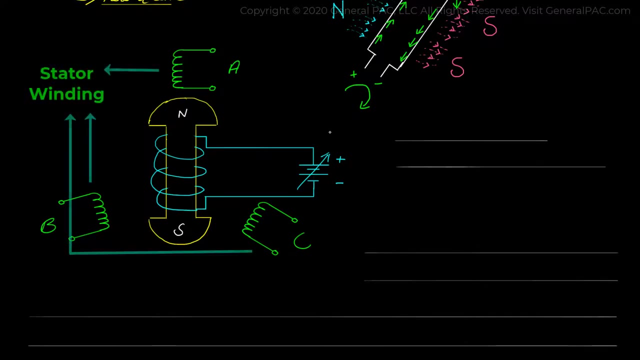 That is, a conductor moving in a constant magnetic field would experience a voltage induced on it. Now, after having a brief idea on Motional EMF, now let's move on to the discussion about how motors work using these concepts. In an AC machine, three-phase stator windings are placed in rotor-conductor. 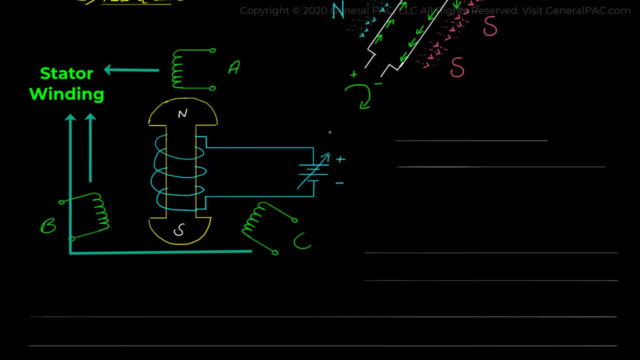 The voltage provided to the stator winding produces the required rotating flux. The rotating flux, or the magnetic field, cuts through the rotor bar and induces an EMF in the rotor. The current that is set up in the rotor bars tends to produce its own magnetic field. 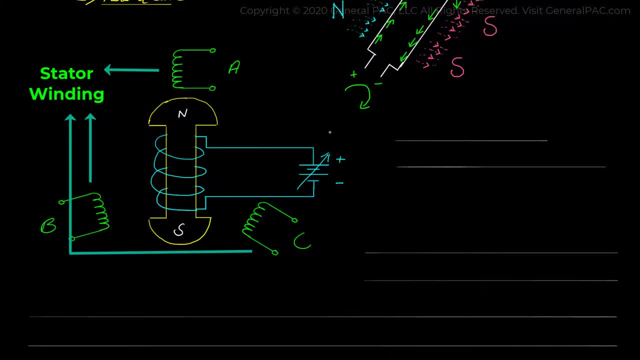 that tries to catch up the rotating magnetic field produced by the winding The rotor gets the torque needed to rotate and can be seen through the torque formula for AC machines, which links the magnetic field of the rotor and the stator with the torque. Now, this is the equation. T is the torque. 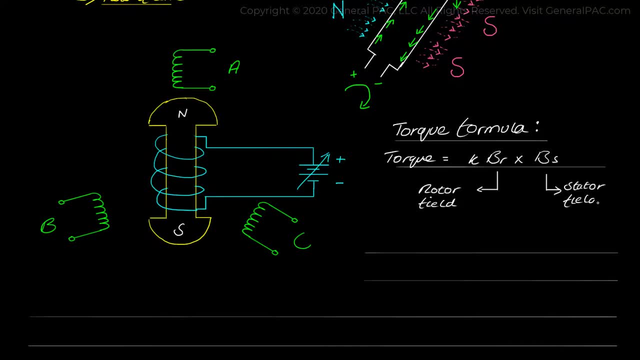 Br is the rotor magnetic field and Bs is the stator magnetic field. The formula explains that in order to have a torque set up, it is required to have both magnetic field in the rotor and the stator to be present and, as we stated before, or else there is no rotation of the rotor. 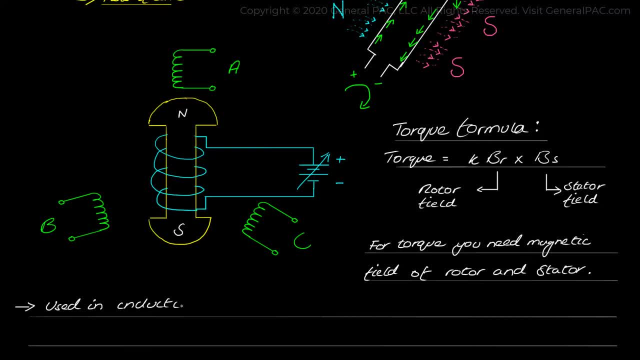 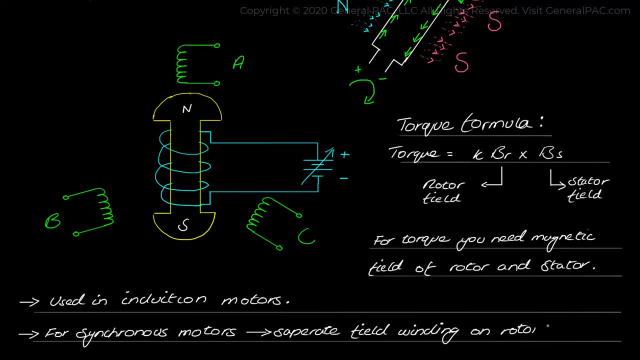 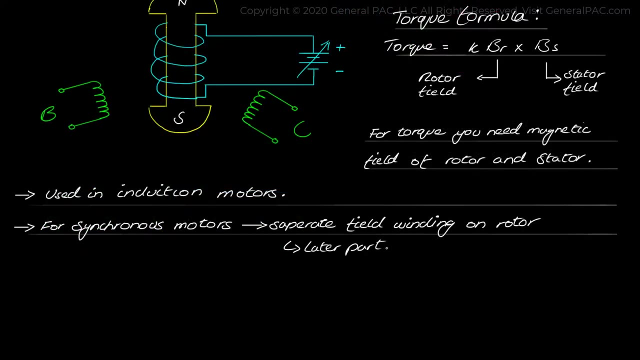 This phenomenon is used in AC induction motors and for synchronous motors there is a separate field winding on the rotor to create the magnetic field that follows the rotor. We will look at synchronous motors in more detail in later part. That's all for this part. 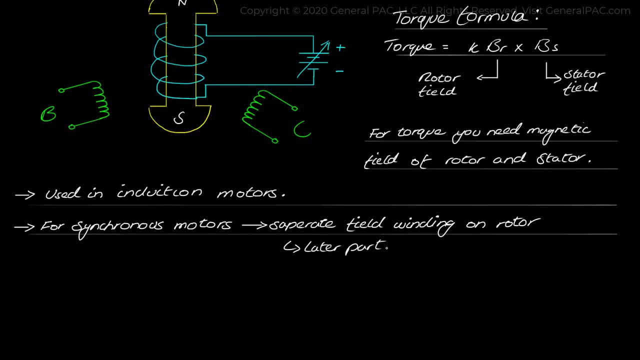 In the next video, we will look at induction motors in detail. We hope that you have a continued interest in this topic and in this series, as either a student or a professional, and we also hope that you find this content useful and enlightening. Please consider subscribing to GeneralPACcom. 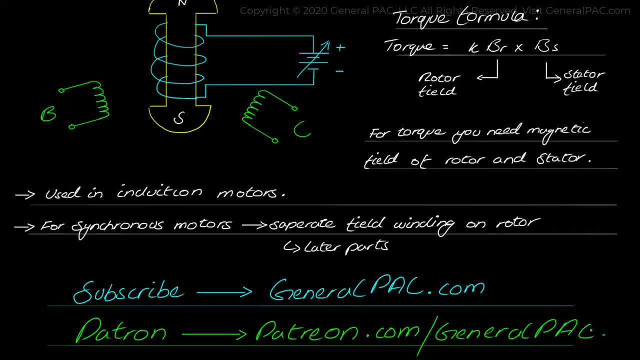 or becoming a patron at patreoncomgeneralpaccom Make making power systems intuitive, open and free to everyone, everywhere.